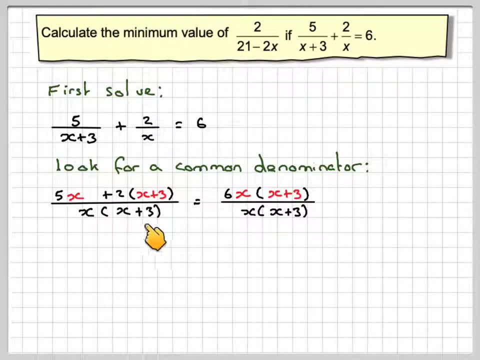 Right now because we've got a common denominator. okay, we don't need to worry about the denominator anymore. So we now expand the numerator. Note: you no longer need the denominator. So that's going to be 5x plus 2 times x, which makes 2x, plus 2 times 3, which makes 6.. 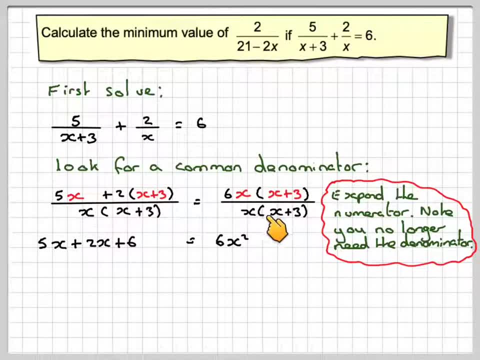 And here we're going to get 6x squared plus 18x. This is a quadratic. In order to solve a quadratic, we need to put it equal to 0. So we'll just collect these two terms together. 5x plus 2x is 7x plus 6, which is equal to 6x squared plus 18x. 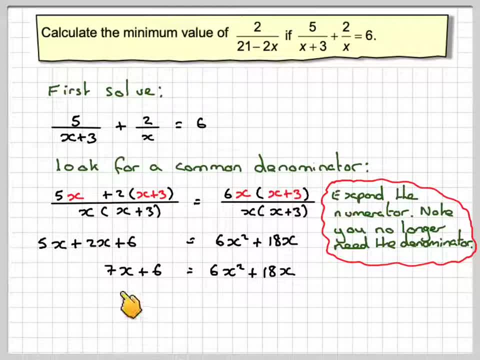 Remind you not to do too much. So we're going to take 7x. So 18x takes 7x gives me 11x, and then we're going to take 6 as well. It'll be equal to 0.. So we need to solve that quadratic. 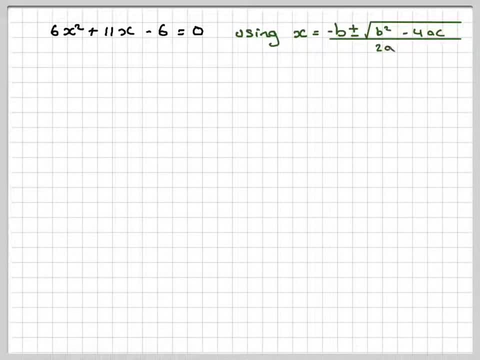 It doesn't factorise so we'll have to use the quadratic formula. So it's worth learning the quadratic formula. So minus b, plus or minus the square root of b squared minus 4ac over 2a Right under here: ax squared plus bx. 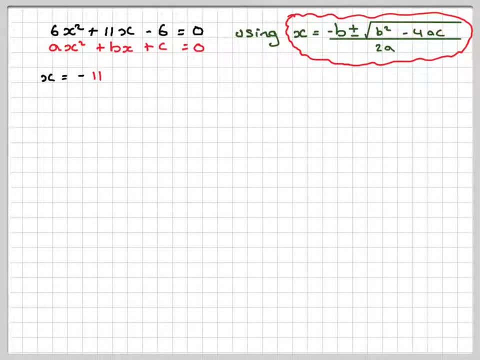 That means x will be equal to minus 11 because b is 11.. So minus 11 plus or minus 11 squared b, squared minus, 4 times 6 times c. But notice anything negative. you should put it into brackets: All over 2 times a, which is 2 times 6.. 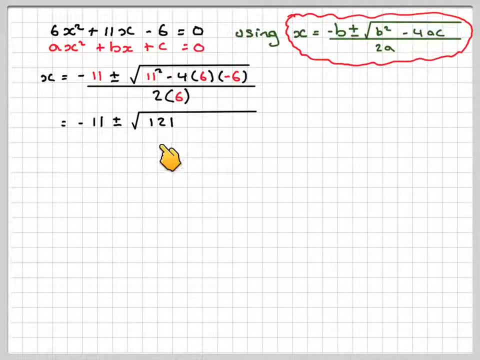 So it's going to give minus 11, plus or minus Square root of 121, 11 squared. This will be plus because you've got a minus times a minus 4 times 6 times 6 is 144.. Minus minus makes it plus. 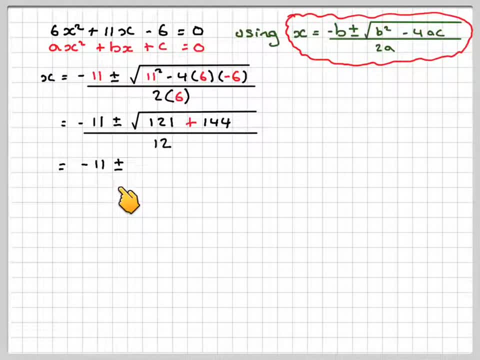 All divided by 12.. So we're going to get minus 11, plus or minus the square root of 121 plus 144, which is 265.. Divided by 12.. Now we're going to use our calculator. Now, on our calculator, we make sure we use the fraction button.